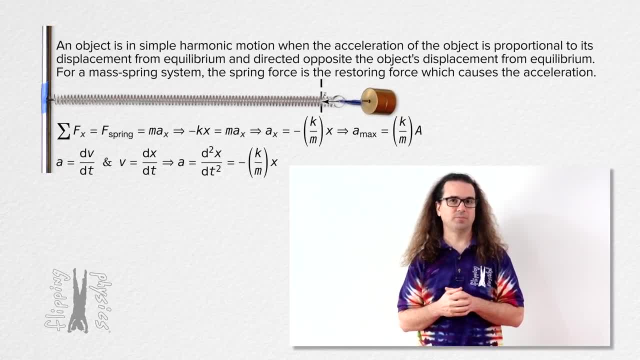 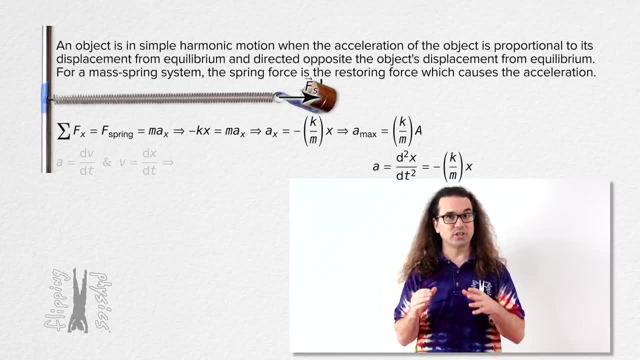 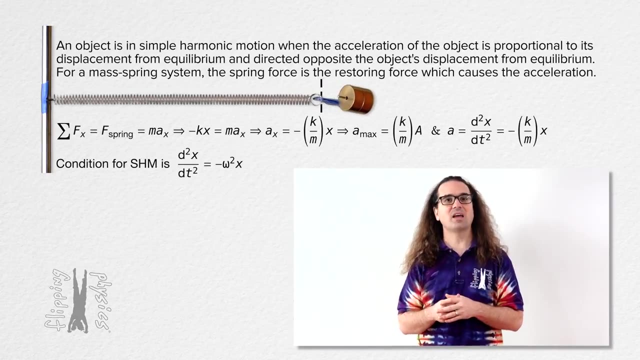 And we can now substitute that into our previous equation. Now this equation gives us the general idea of the mathematical definition of simple harmonic motion, which is that the second derivative of position with respect to time equals the negative of omega squared times position where omega is called n. 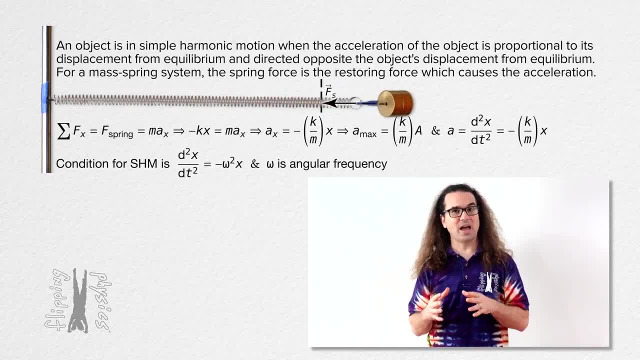 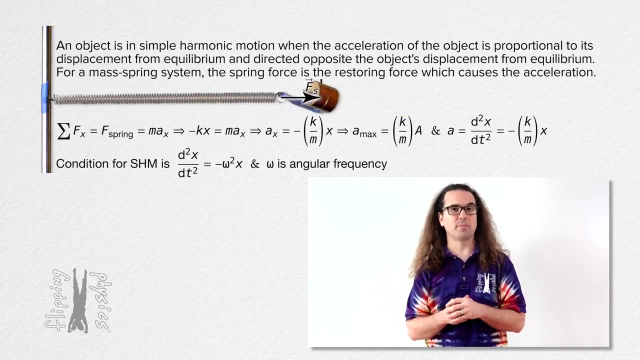 This equation describes simple harmonic motion. Notice: the acceleration is proportional to displacement from equilibrium and the acceleration is directed opposite to the direction of the displacement from equilibrium, which are the conditions for simple harmonic motion For a mass-spring system. you can see that the square of the angular frequency 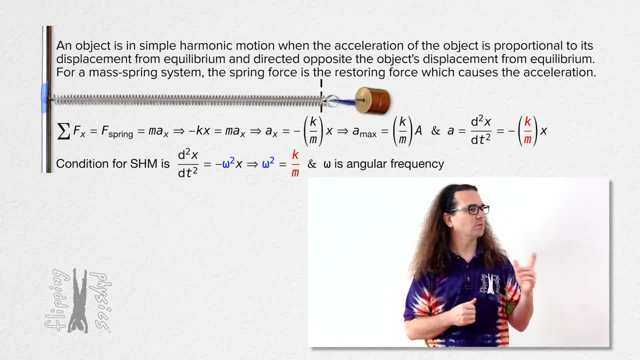 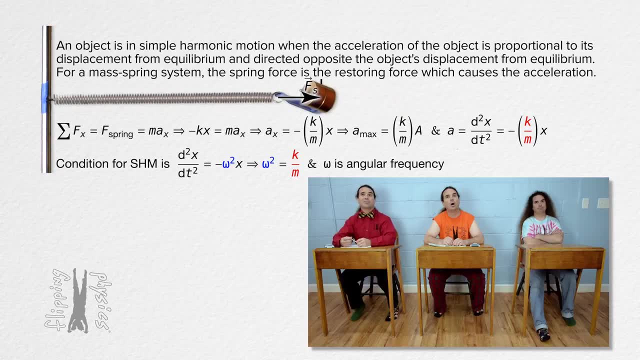 equals spring constant over mass. Mr P. Yes, Billy. Why is the square of the angular frequency equal to the spring constant over mass? That is a fair question, Billy. I will show why that is in just a bit. We're not quite there yet. 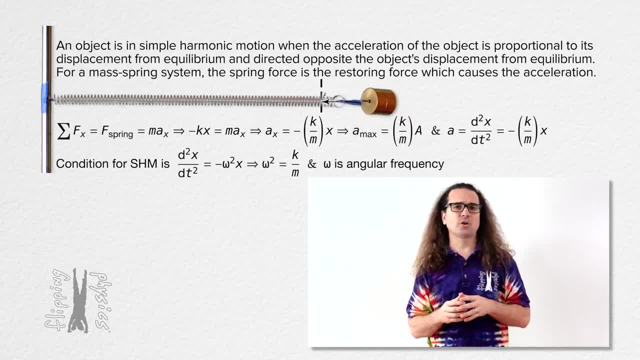 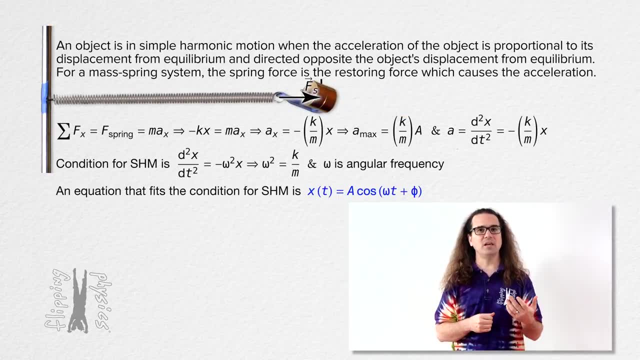 Okay, Yeah, A position equation which satisfies the mathematical definition of simple harmonic motion is: position as a function of time equals amplitude times, the cosine of the quantity. angular frequency times, time plus phi the phase constant- Billy, remind me of what phi the phase constant is. 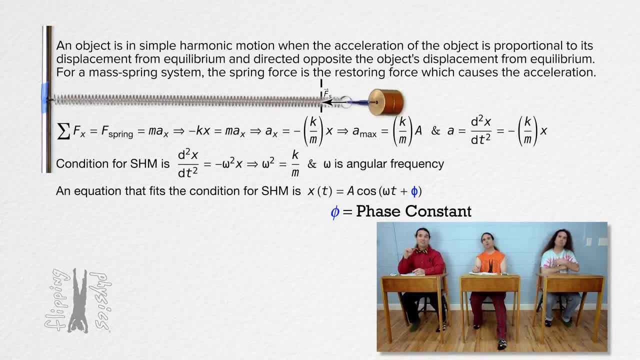 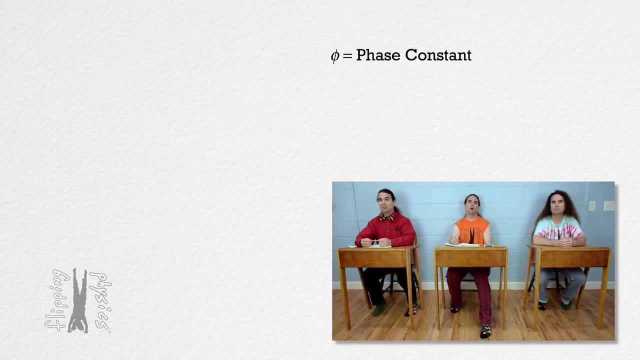 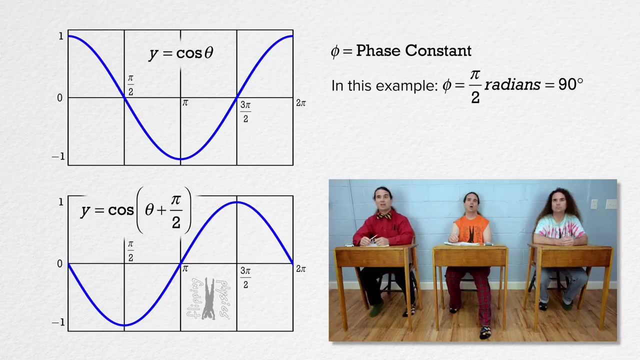 Absolutely. Phi is the phase constant or the phase shift for the wave. For a simple example, we can look at the graph of y equals cosine theta with theta in radians and compare that to the graph of y equals the cosine of the quantity theta plus a phase constant of pi over 2 radians. You can see: 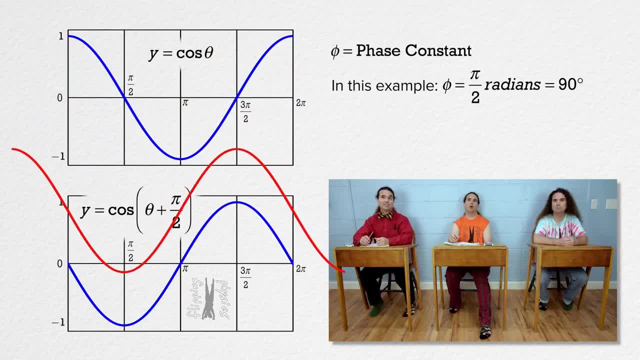 that the cosine graph is phase shifted to the left by the phase shift to the right of the wave. So y equals pi over 2 radians, which is also 90 degrees. That is what the phase constant does. It shifts the location of the cosine or sine wave along the horizontal axis. 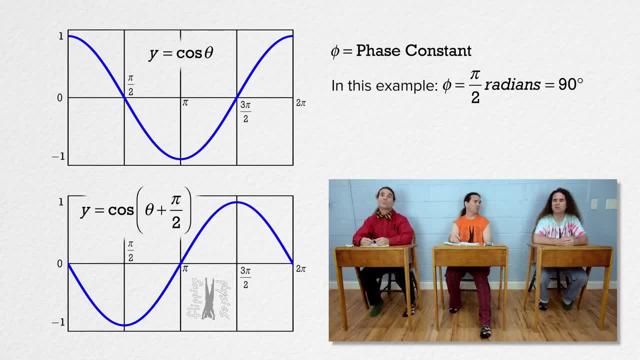 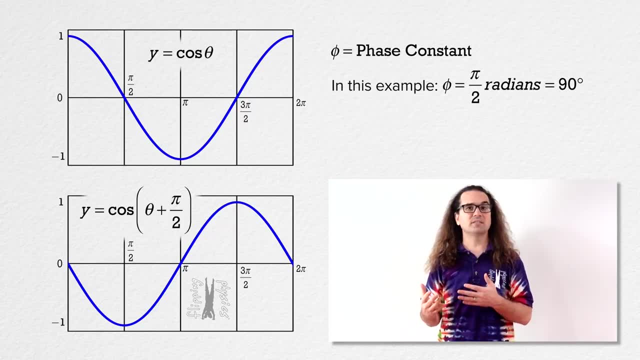 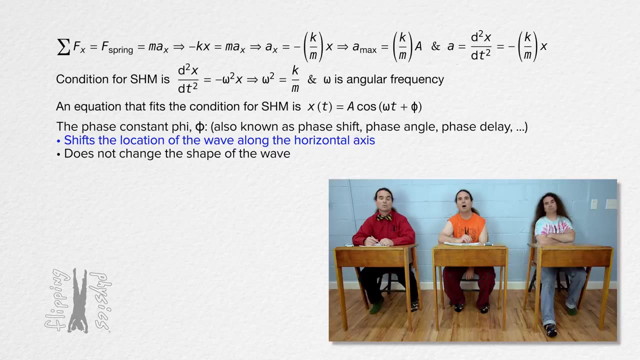 I thought phi was the phase angle. I've heard it is called phase delay. Yeah, phi has a lot of names. Most often I have heard it called phase constant or phase shift. The most important thing to know is that it shifts the sine or cosine wave along the horizontal. 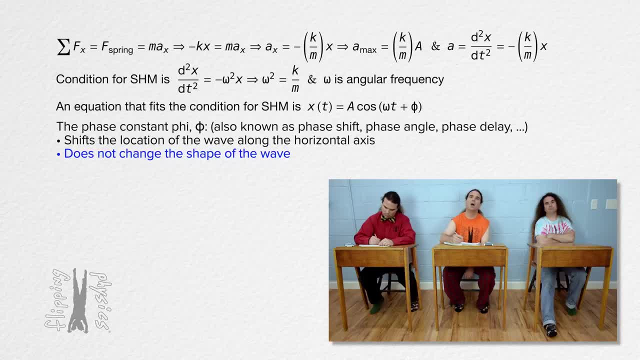 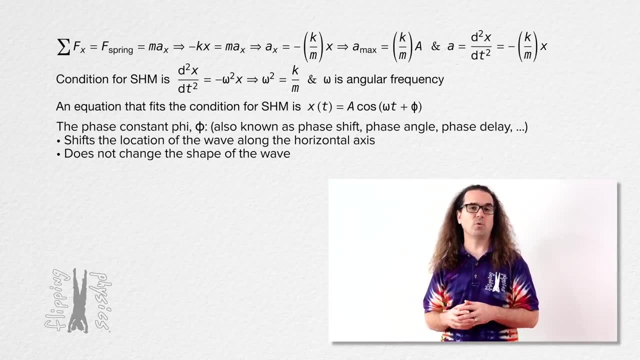 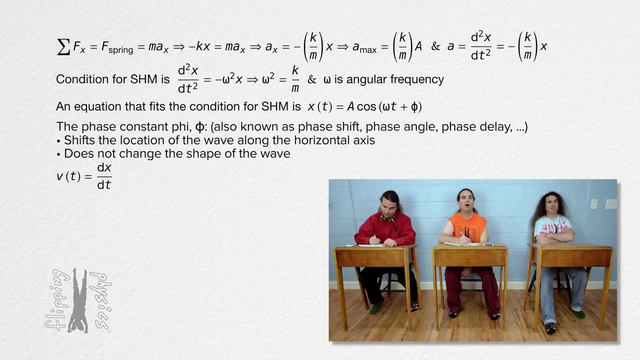 axis. However, it does not change the shape of the wave. Bo. please determine the velocity of an object in simple harmonic motion using the position equation. Well, velocity equals the derivative of position with respect to time, So the derivative of the position equation with respect to time. Amplitude is constant, so that comes out of the. 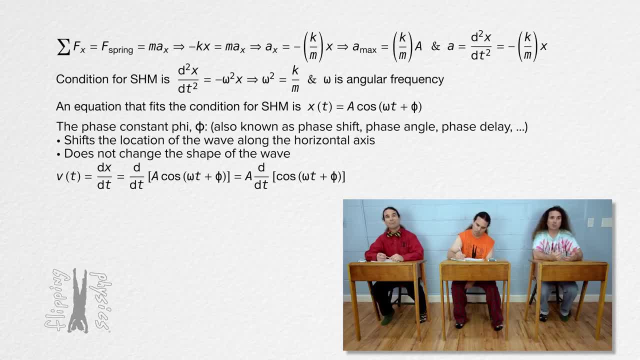 derivative. We need to use the chain rule. So the derivative of cosine is negative, sine The same quantity as before, And then the derivative with respect to time of that quantity, or angular frequency times, time plus phi. The derivative of that with respect to time is: 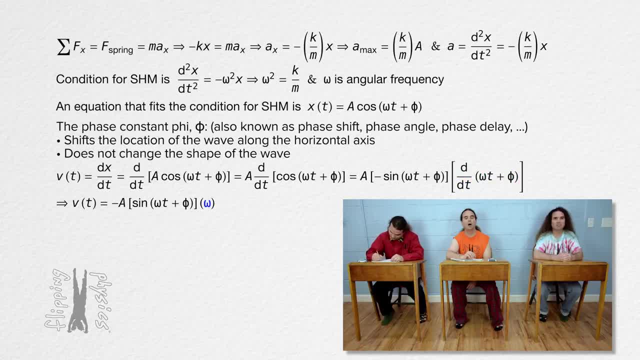 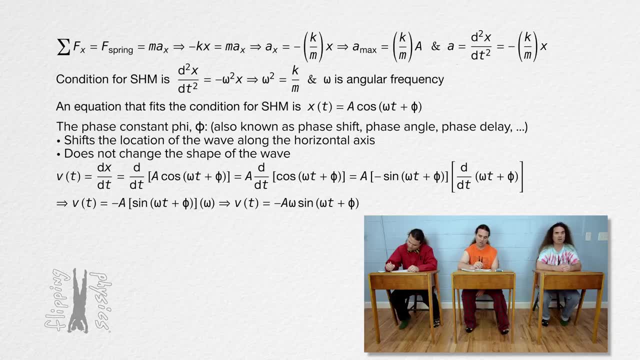 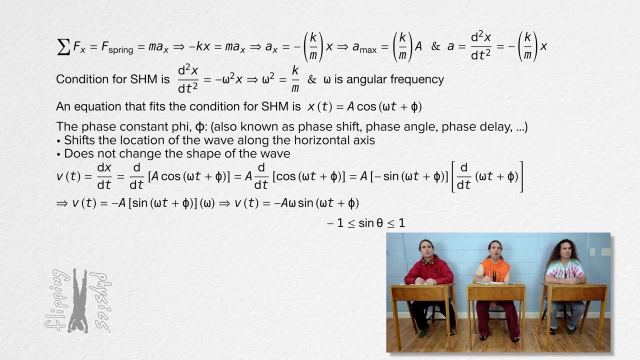 just angular frequency. So velocity of an object in simple harmonic motion with respect to time equals negative amplitude times angular frequency, times the sine of the quantity, angular frequency times time plus phi. And what then is the maximum velocity equal to? Uh, the value of sine theta has a minimum of negative one and a maximum of positive one. 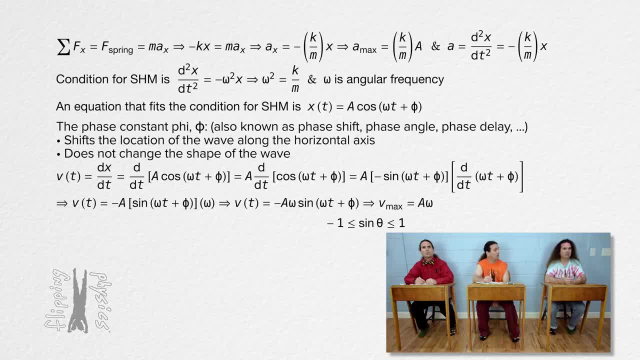 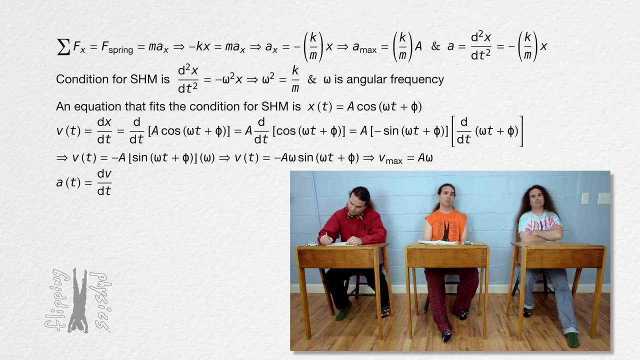 So the maximum velocity equals amplitude times angular frequency. That is correct, Bo. Thanks, Bobby. please determine acceleration as a function of time. Sure, Acceleration equals the derivative of velocity with respect to time. So the derivative with respect to time of the equation Bo just derived. This is: 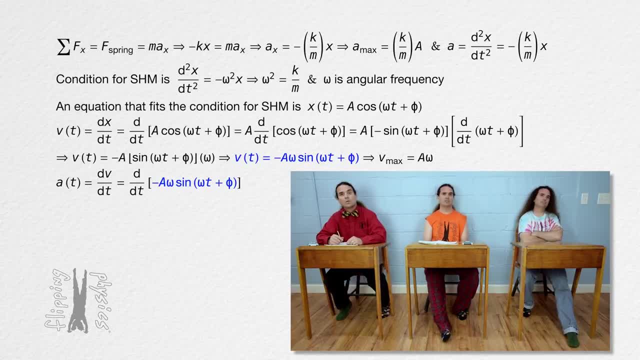 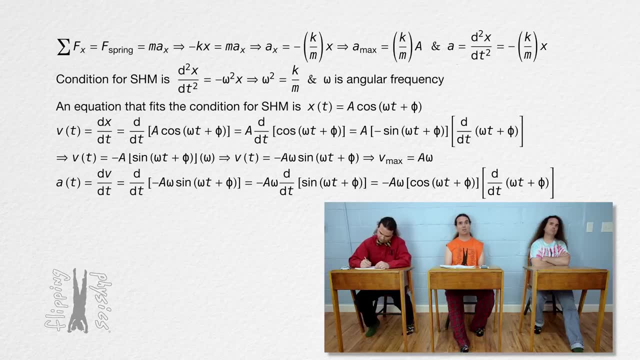 very similar to what Bo just did: Negative amplitude times. angular frequency is constant over time, So take that out from the derivative. The derivative of sine is cosine And we need to use the chain rule Again. the derivative of that parenthetical expression with respect to time is: 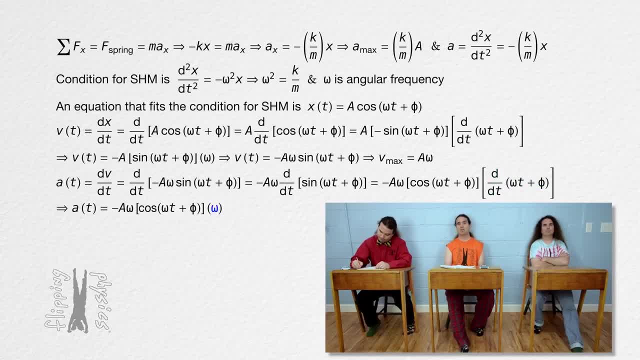 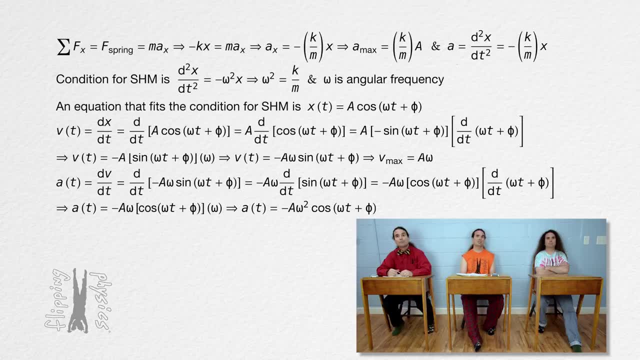 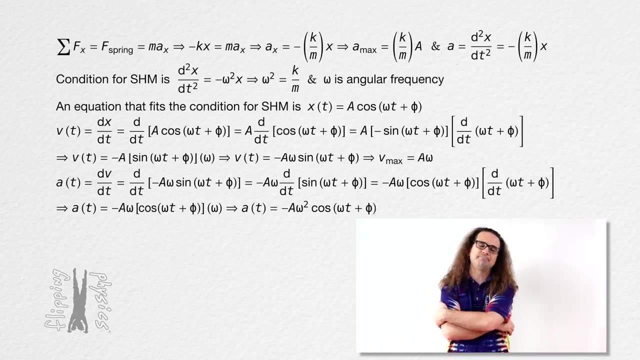 just angular frequency. So the acceleration of an object in simple harmonic motion equals the negative of amplitude times angular frequency, squared times the cosine of quantity, angular frequency times time plus phase constant. And because the value of cosine theta varies between negative 1 and 1,. 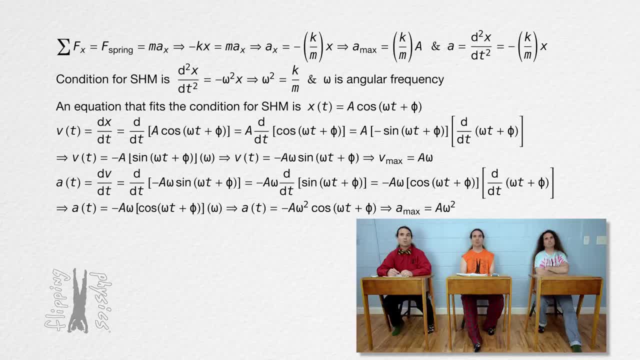 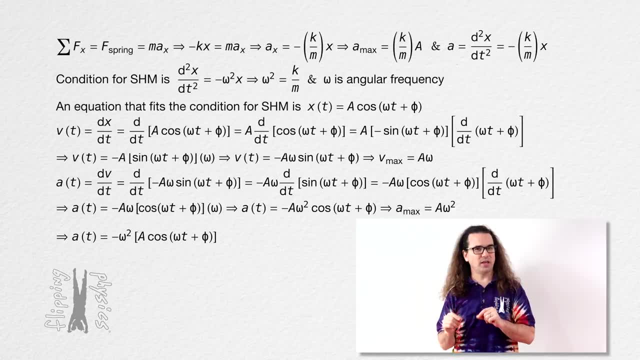 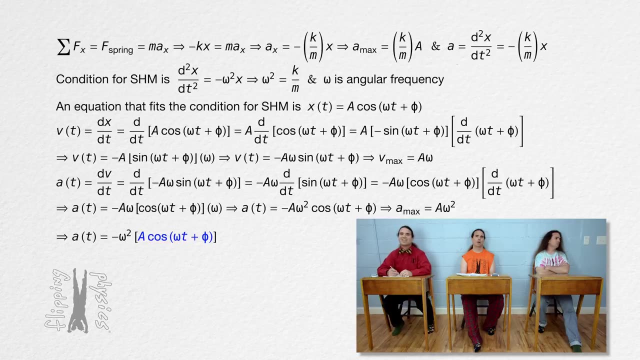 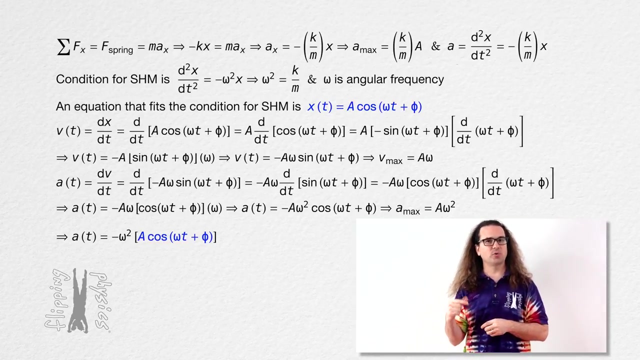 the maximum acceleration equals amplitude times angular frequency squared. Well done, Bobby. Now who can tell me what they see when I rearrange the equation slightly? What is between the brackets in the acceleration equation? That is the position equation. Correct, Billy? That means we have just shown that this position equation satisfies the conditions. 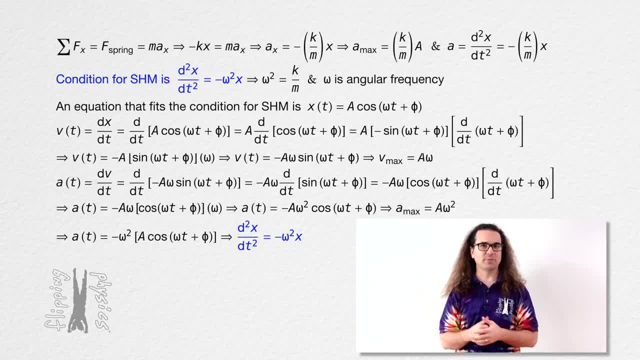 for simple harmonic motion, The second derivative of position with respect to time equals the negative of the square of angular frequency times position. Cool, Yeah, Huh. And now we can see why the equation for simple harmonic motion has the square of angular frequency in it and not just angular frequency. 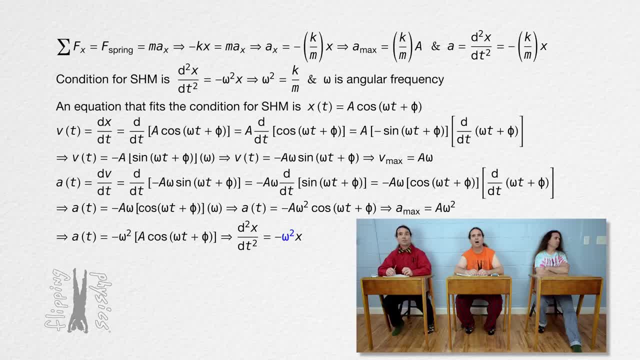 Oh right, I see it. It is because when we start with that equation for position and take the derivative of it with respect to time twice, we get: acceleration equals the negative of the square of angular frequency times position, The square of angular frequency. 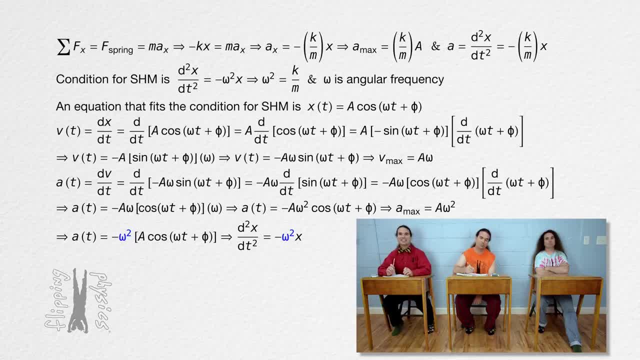 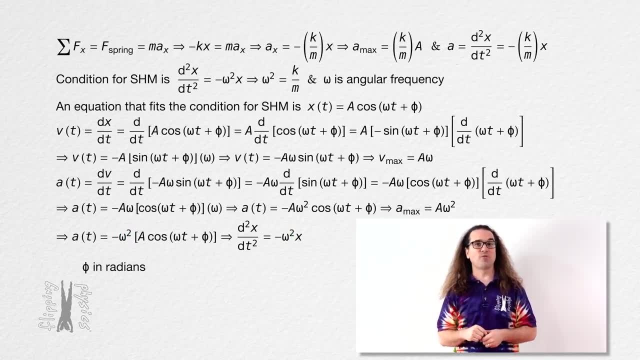 is right there in the derivation of the acceleration equation. Exactly, Billy. Thanks, You are welcome. Please remember to use radians for phi, the phase constant, and radians per second for angular frequency. Actually, let's talk some more about angular frequency. 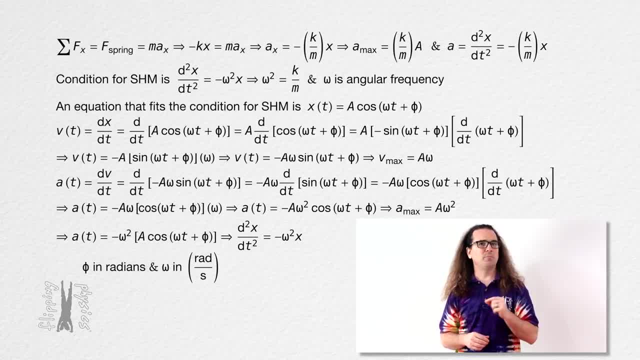 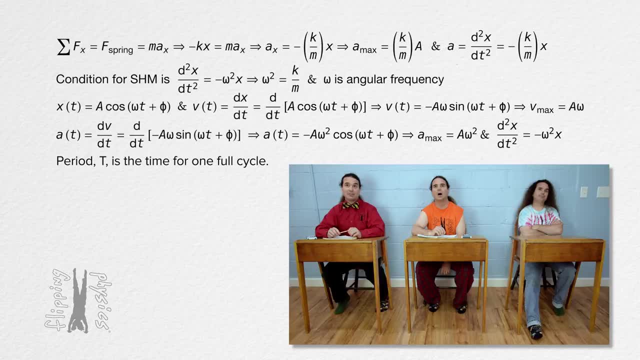 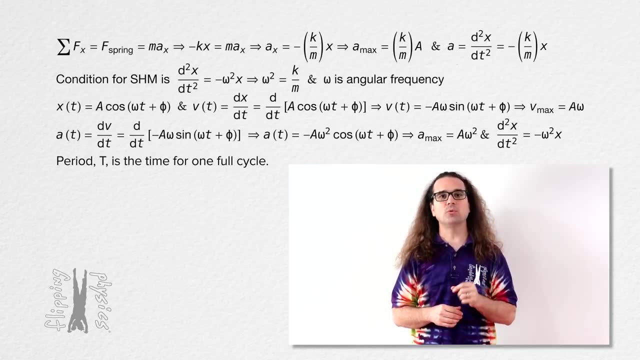 starting with period Billy, what is the period of simple harmonic motion? In simple harmonic motion period, capital T would be the time interval it takes for an object to go through one full cycle. In other words, the values of the position equation should be equal. 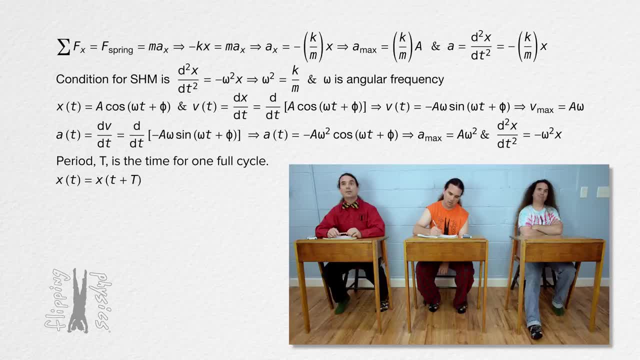 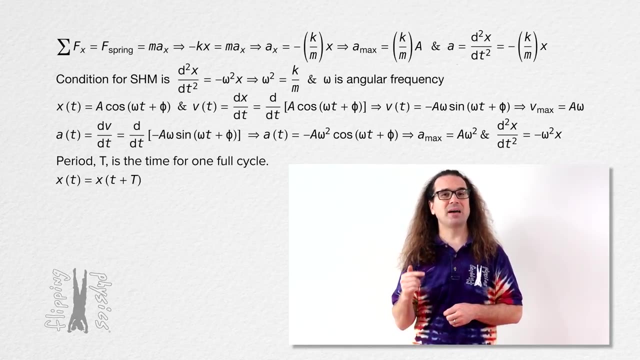 at times t and t plus the period Right After one full cycle the position is the same, so the position function should give equal results after time t and time t plus the period. That makes sense. Also, after one full cycle, the phase has increased by 2 pi radians. 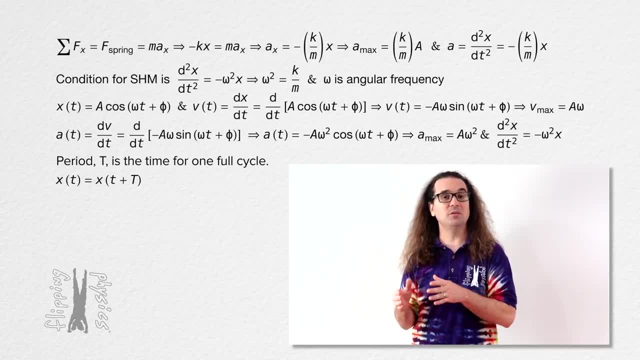 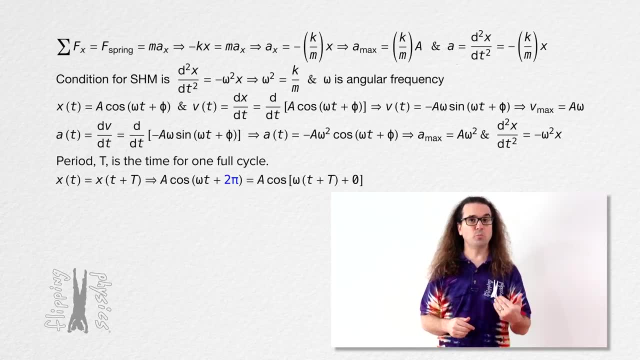 In other words, the position at time t equals the position at time t plus the period Substituting in the equation for position. in both cases, for time t, the phase shift will be 2 pi, and for time t plus the period, the phase shift will be zero. 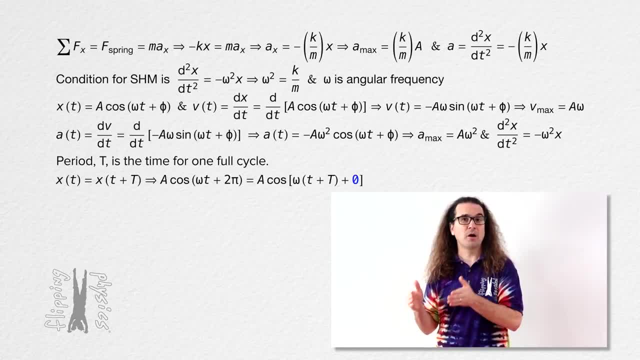 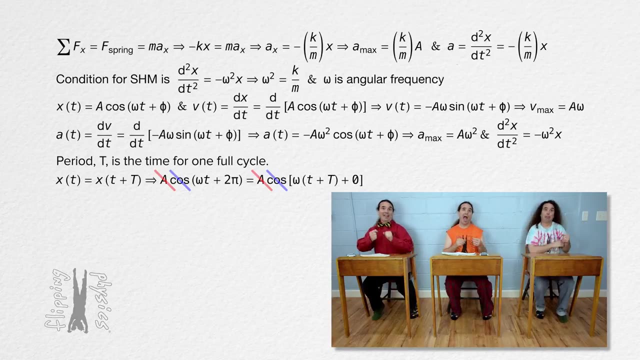 In other words, we need to shift the wave forward by 2 pi radians at time t in order for the position to be exactly equal at time t and time t plus the period And… Everybody brought amplitude times cosine to the party. Technically, we have to take the inverse of cosine of the whole equation. 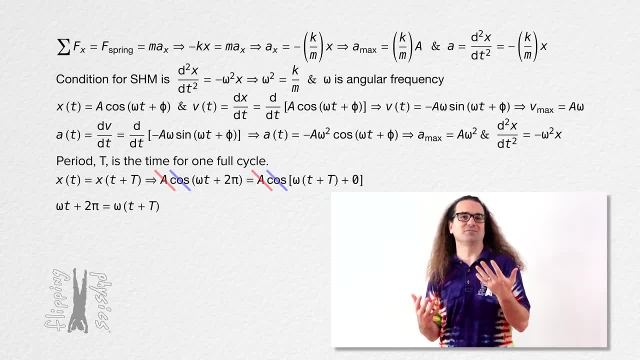 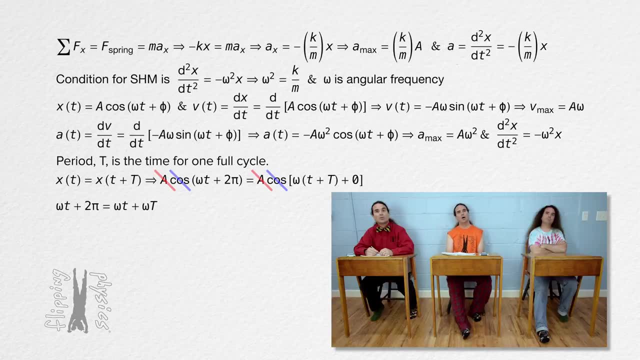 but sure everybody brought amplitude times cosine to the party, Close enough for dancing …. …, …, … … … … And when we multiply through by omega on the right-hand side, you can see we can subtract angular frequency times time from both sides. 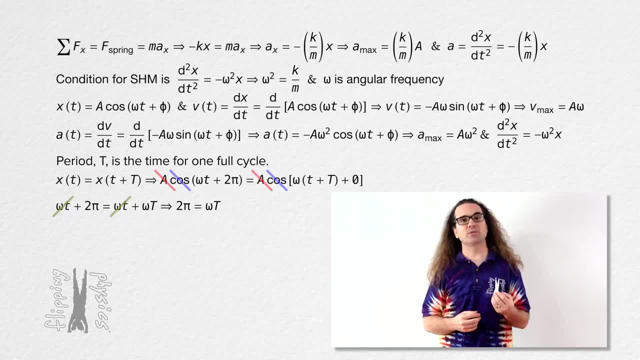 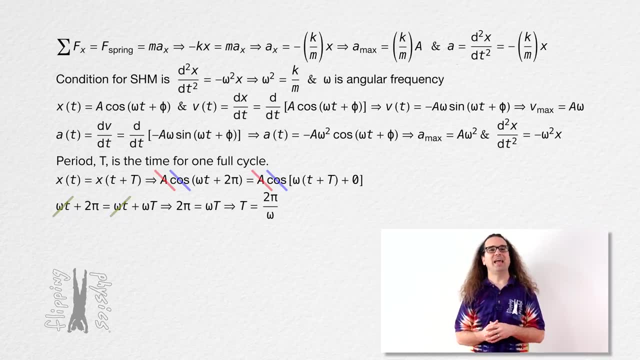 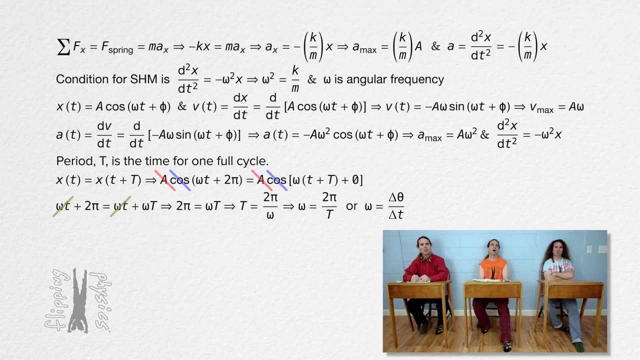 Sure, That leaves us with 2 pi equals angular frequency times period. Therefore, period equals 2 pi divided by angular frequency or, if you prefer, angular frequency equals 2 pi over period. Before we just used angular velocity equals angular displacement over change in time. 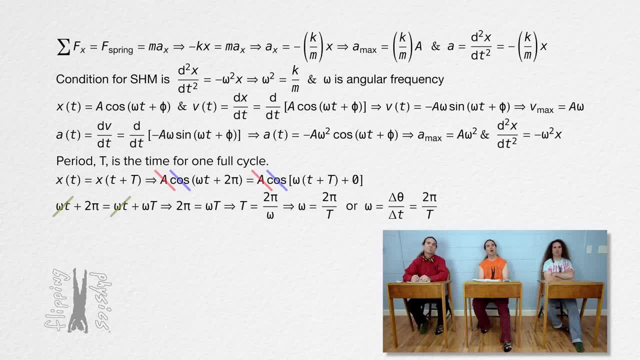 For one full cycle, that equals 2 pi over time. True, but the way I just did it does not use the equation for angular velocity. Oh … … … … … … … …. Right, And that makes it more clear that omega in these simple harmonic motion equations is: 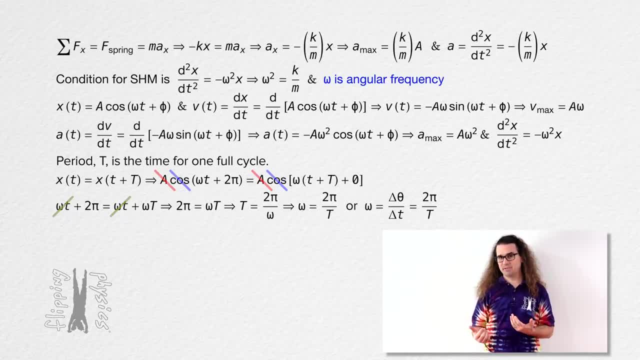 angular frequency. Honestly, I do not have a preference of which way you use to determine the equation for angular frequency. I just think it is useful to understand both derivations of angular frequency. Speaking of frequency, frequency equals the inverse of the period. therefore, angular frequency equals 2 pi times. 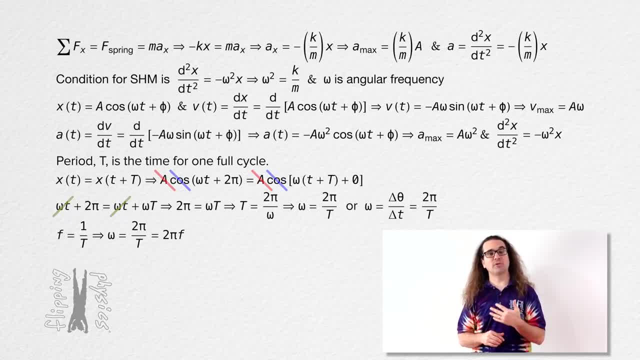 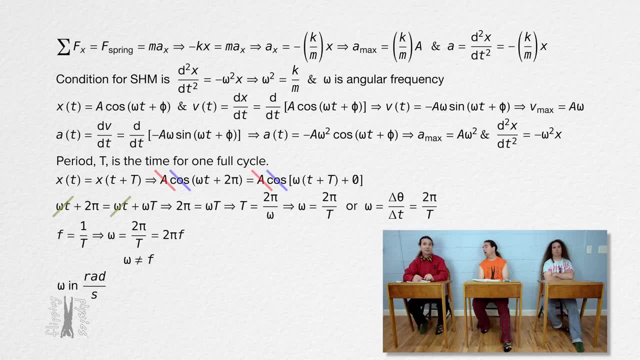 frequency, which illustrates that angular frequency and frequency are not the same, And the units for angular frequency are radians per second. however, the units for frequency are 1 over seconds or cycles per second, so even their units are different, Correct, Billy? 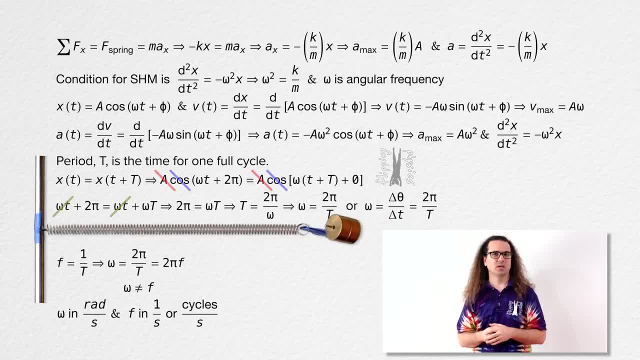 And now let's return to the mass spring system. If you recall, we derived that the angular frequency of a mass spring system equals the square root of the spring constant over mass. We can now substitute that into the equation we derived for the period of simple harmonic motion. 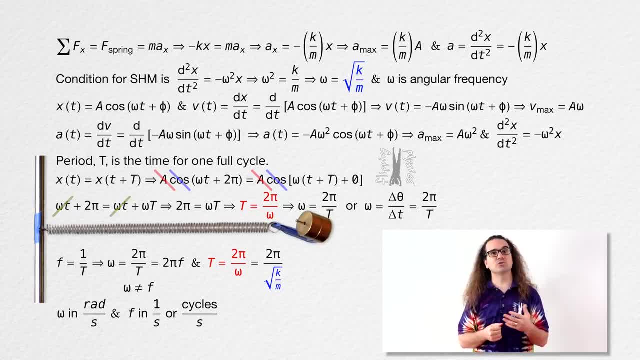 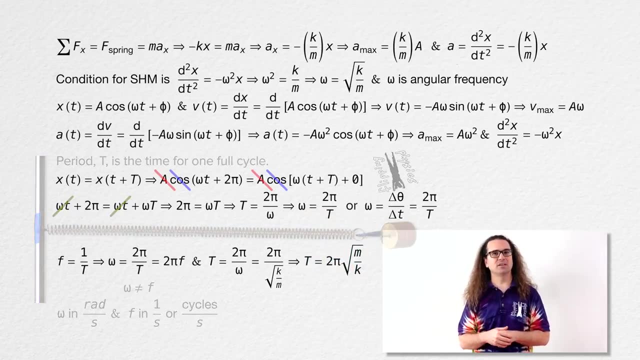 and show that the period of a mass spring system equals 2 pi times the square root of mass over spring constant. We have used this equation many times before. now we know how to derive it. The main takeaways from today's lesson are that the mathematical condition for simple, harmonic motion